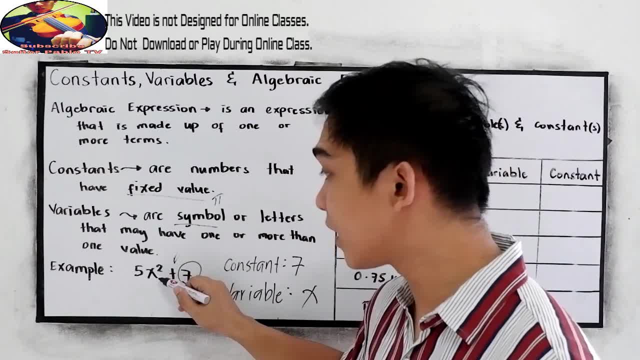 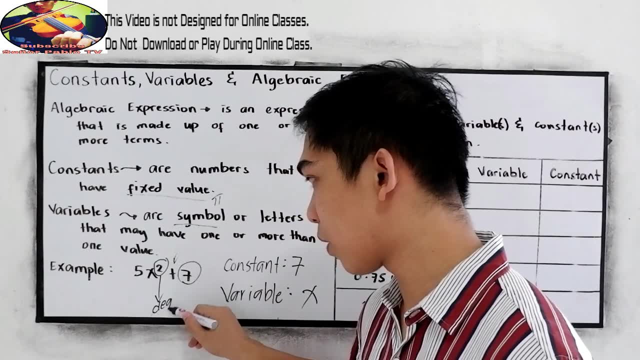 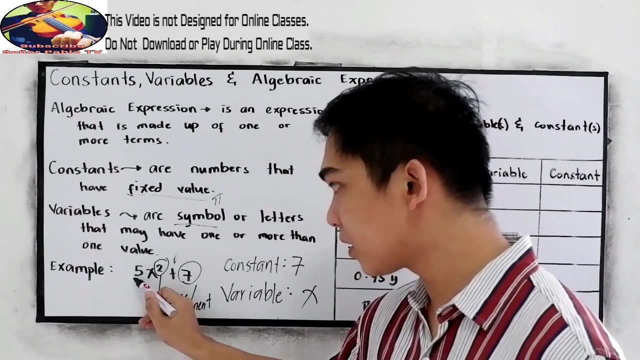 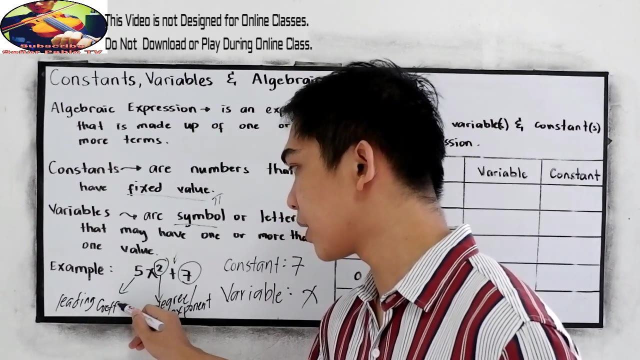 So we have this exponent or degree. So this is in degree 2, or the second degree. This is what we call the degree Or exponent, And the five here is what we call the leading coefficient. When you say leading, it is written on the 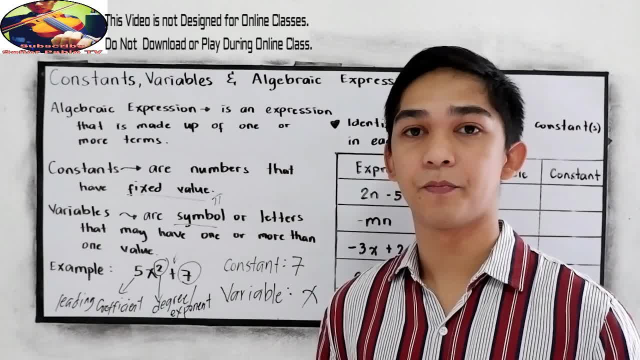 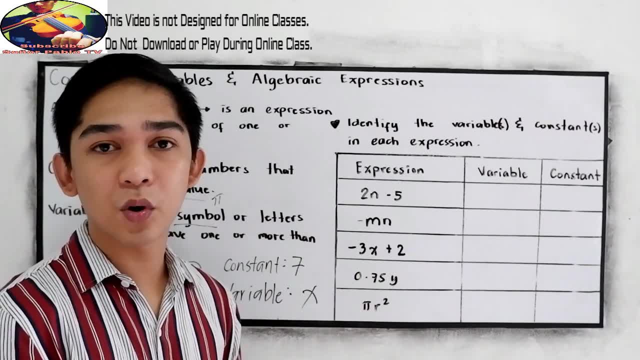 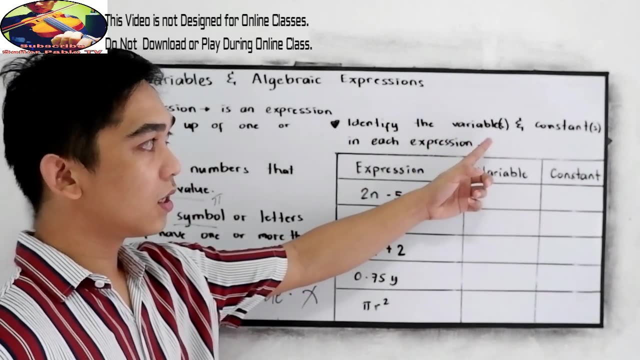 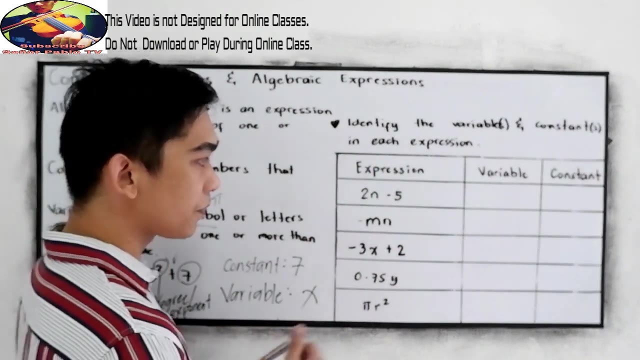 right leg part of our expression. Now let's have this example, Let's see this example. We're going to identify the variable and the constant in each expression. So identify the variable or variables and constant in each expression. So our expression here number one: 2n minus 5.. 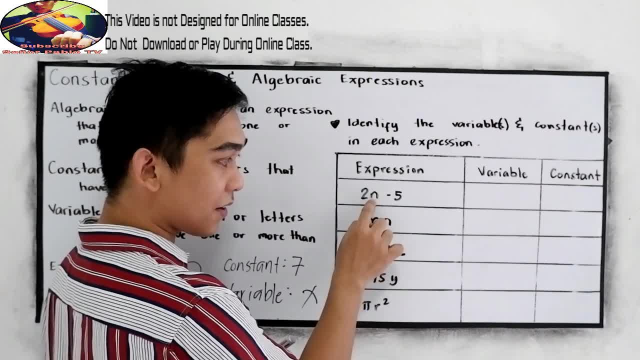 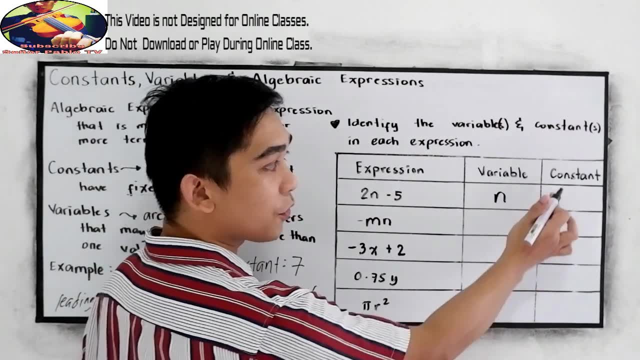 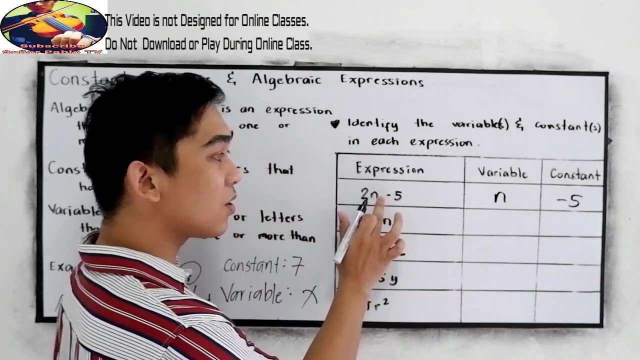 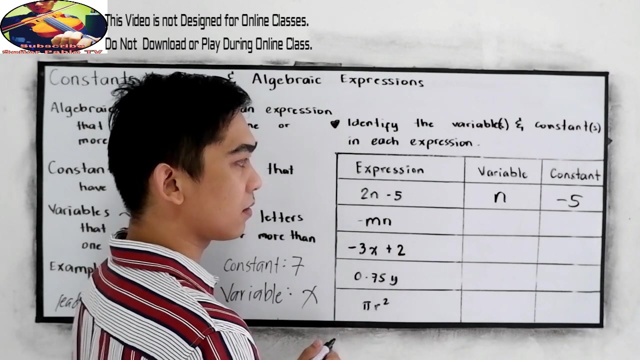 Our variable is. so we have a letter which is n, And for the constant, our constant is negative, 5.. And put the sign of our constant, Next, negative mn, In number two. we have two variables, We have two letters, the m and n. 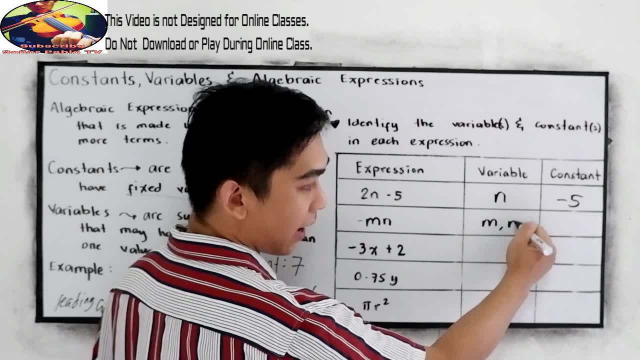 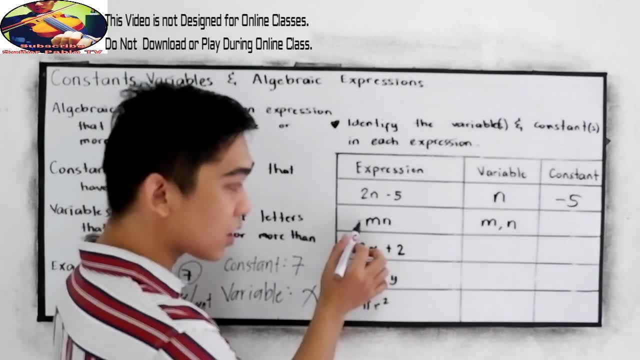 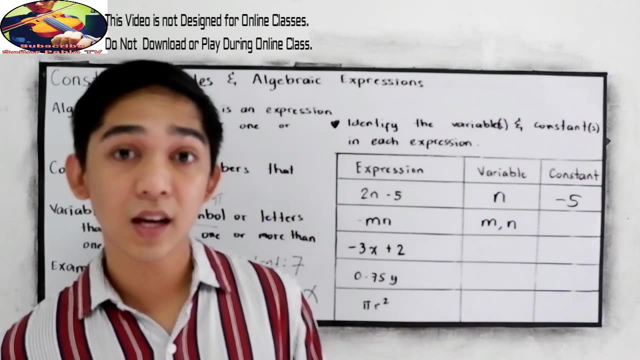 So we're going to write mn. Sir, do I need to write the sign of our m? So notice, we have negative in that. So since we are talking with the variable, there's no need to write the sign in our variable, Just the letter itself. 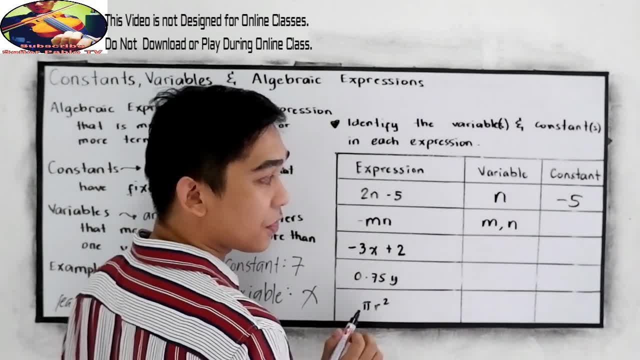 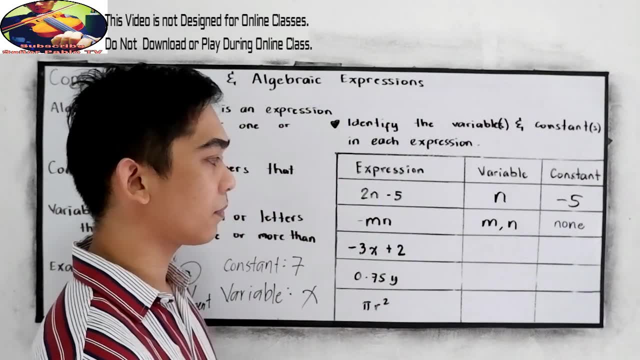 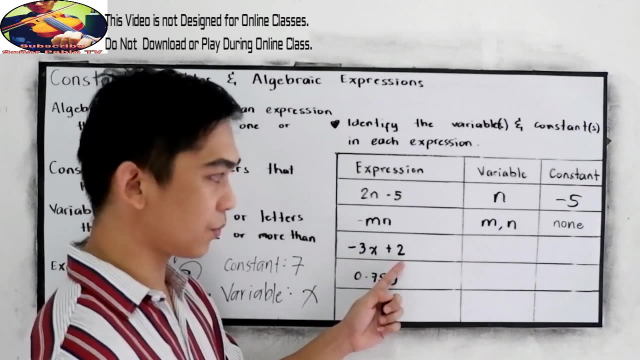 And for the constant term. we don't have a constant term, So we can write here as none. There is no constant term. Next, number three: The given is negative 3x plus 2. So we have a letter which is x.